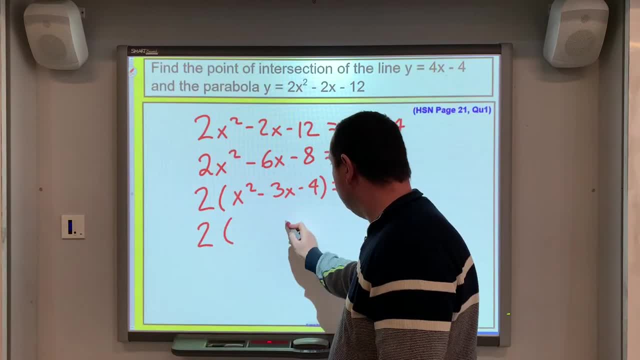 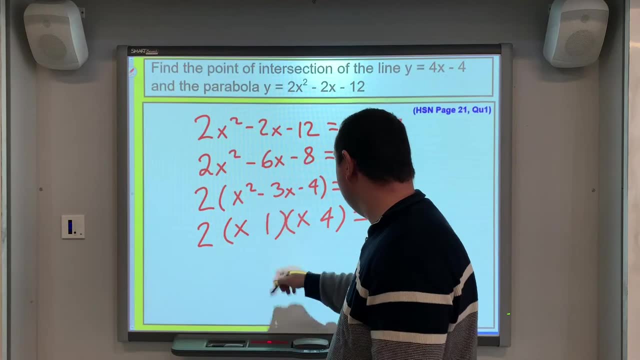 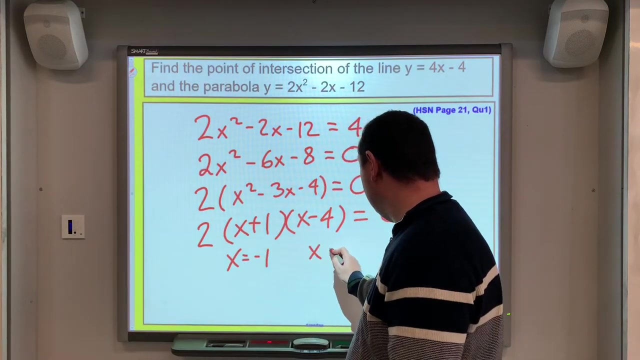 Factorising, we get double brackets: x and x, 4 and 1, minus 4 plus 1 is minus 3.. So x equals minus 1 and x equals 4.. So we've got our x part. We now need to find the y part, because we want the point. 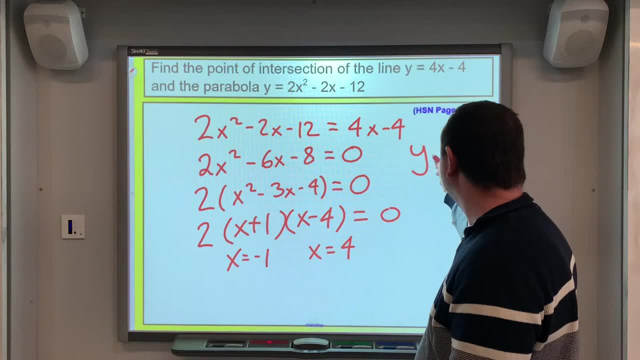 of intersection. But remember, y was equal to 4x minus 4.. So substituting both of them values in For minus 1, we get 4 times minus 1, take away 4, that's minus 8.. So the first. 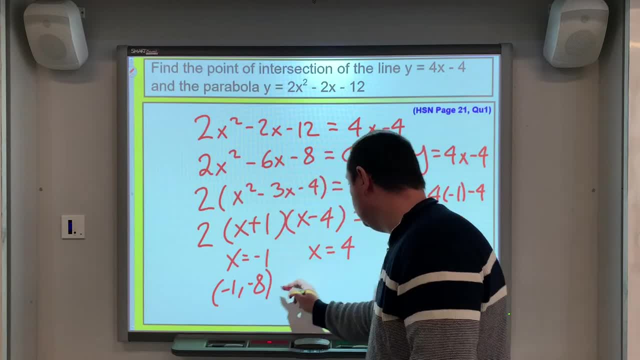 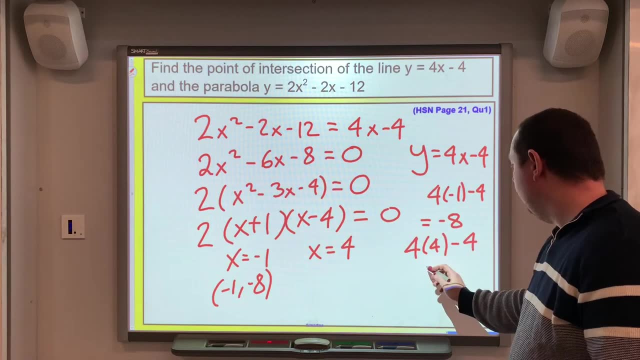 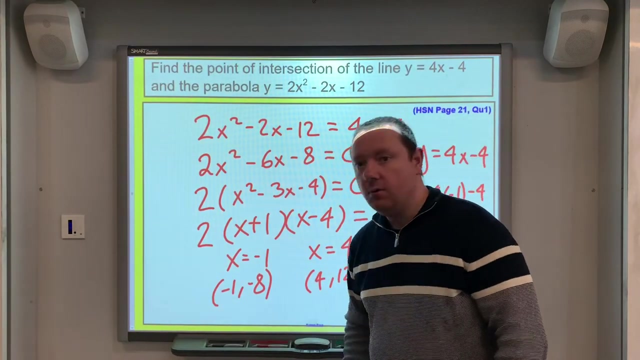 point is: minus 1 minus 8, and substituting 4 into this equation, we've got 4 times 4 minus 4, that's 12.. So the second point is 4, 12, 4.. And we're done. So. example 2 says: 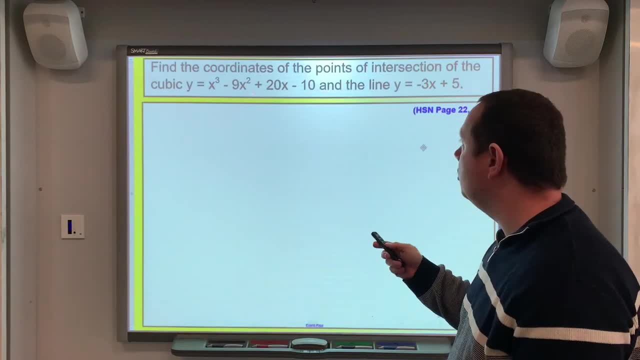 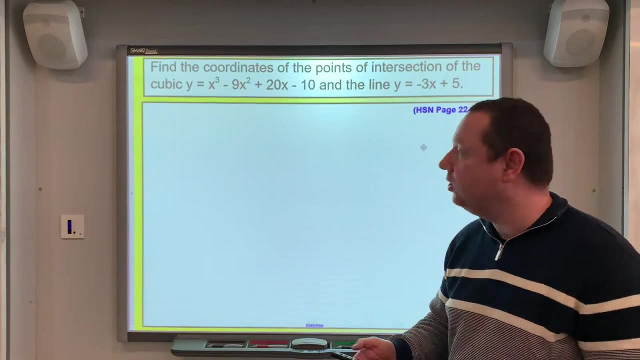 find the coordinates of the points of intersection of this cubic with that equation and this line with this equation. So we're solving them simultaneously because it's the points of intersection. We both say y equals, so we can equate the x side to the other x side. 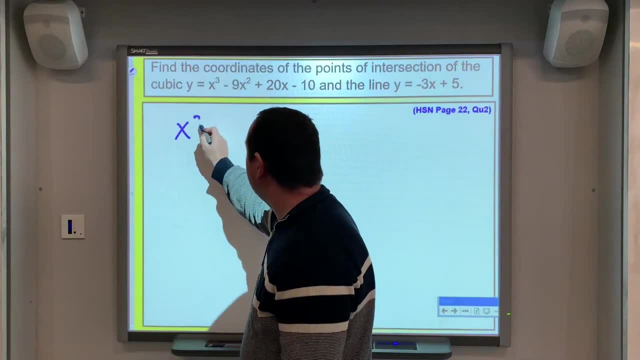 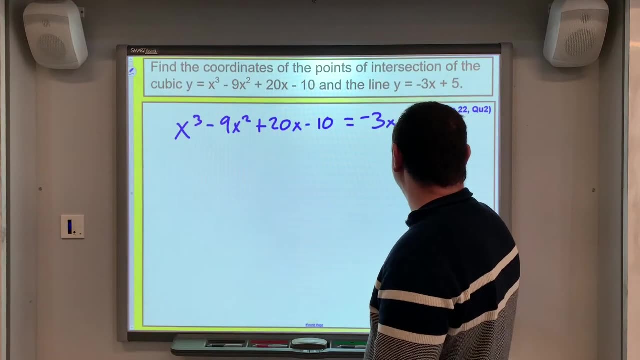 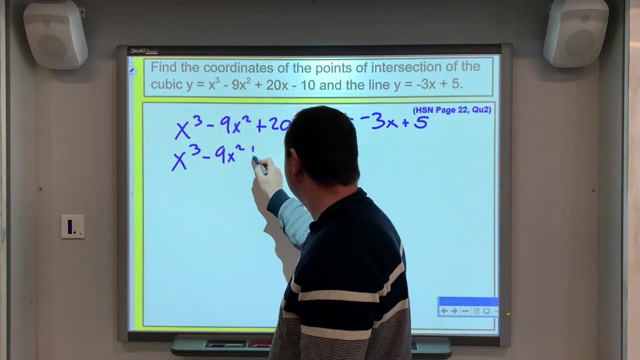 So, writing that up, we get x cubed minus 9x squared plus 20x minus 10, equals minus 3x plus 5.. Taking everything away to the left, we get x cubed minus 9x squared plus 23x minus 15, equals 0.. 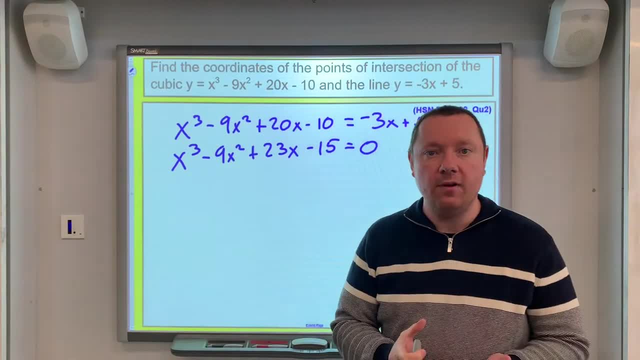 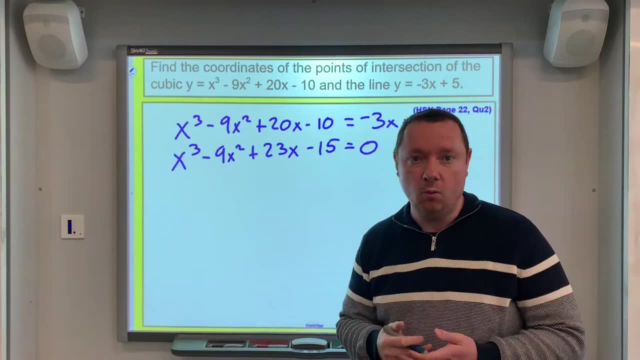 We've got a cubic to solve, so remember to do that we need to find one factor. Once we've found one factor, we can use synthetic division to get the rest. I'm going to immediately use synthetic division and try 1.. So substituting 1 into this equation, we've got 1x cubed minus. 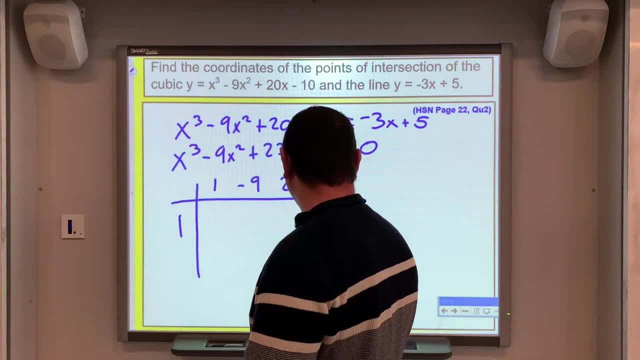 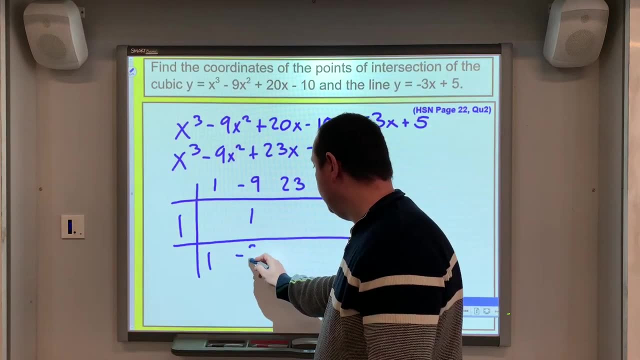 9x squared plus 23x, So we get x minus 15.. 1 times 1 is 1, minus the negative is minus 8.. One times minus eight is minus 8,. 23 minus 8 is 15.. 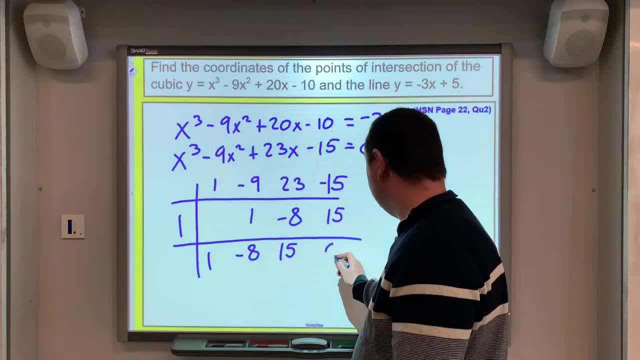 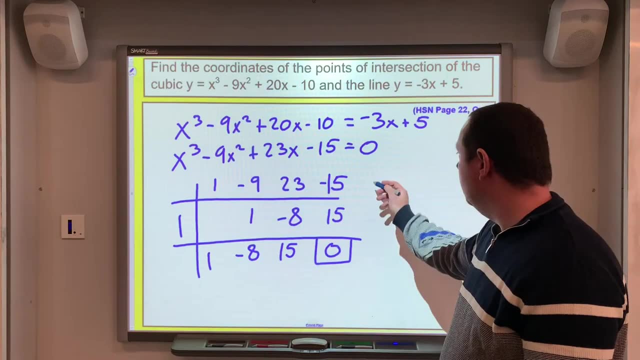 1 times 15 is 15,, 15 minus 15 is zero. Since the remainder is 0, we have found a factor. The factor is x minus 1.. So we know that from this equation here, we're going to have x minus 1, and x squared minus 9x. 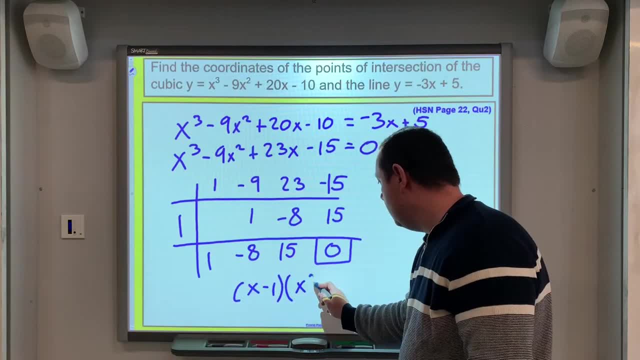 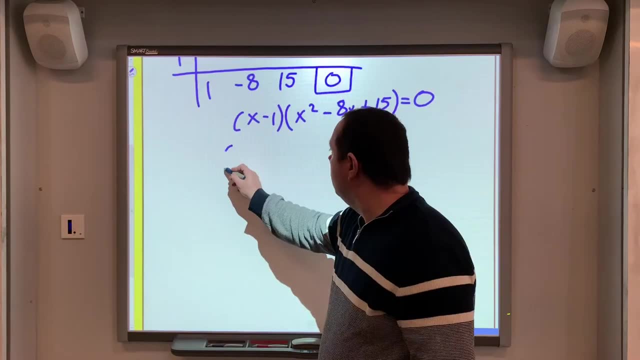 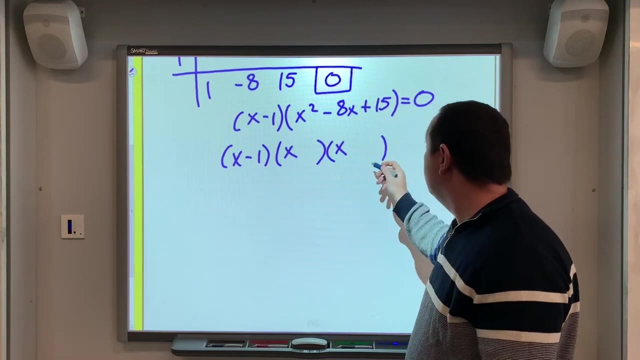 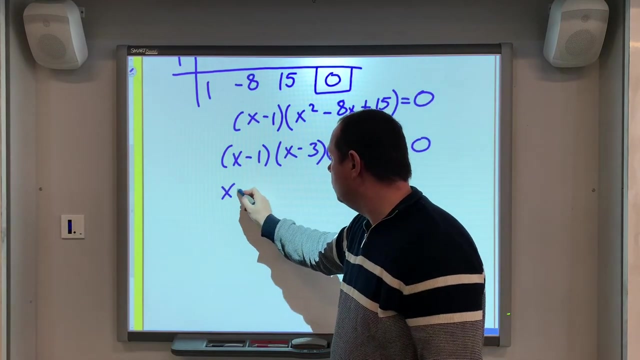 times x squared minus 8x plus 15, and that equals 0.. So that's x minus 1,. double brackets: x and x, 5 and 3, minus and minus. So we've got our three points: x equals 1,, x equals 3, and x equals 5.. 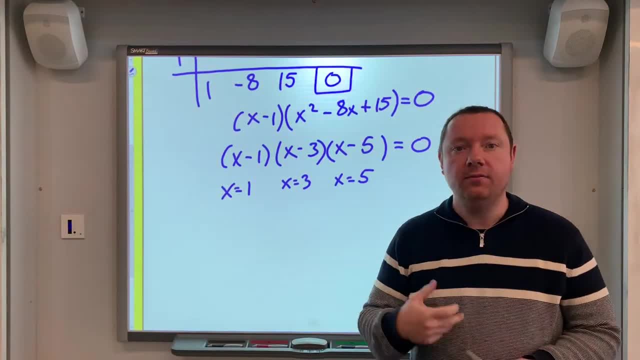 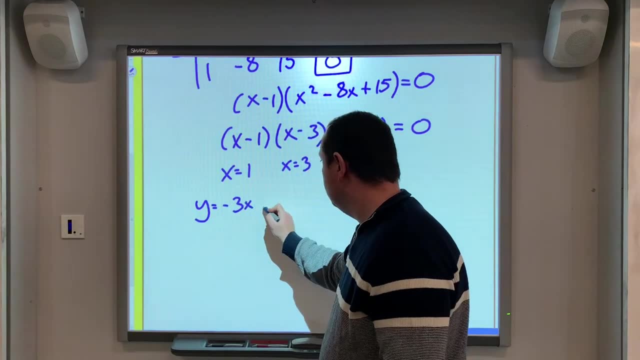 And we need to now substitute that back into y to find the y part. So remember, y was equal to minus 3x add 5, so substituting each of them in. So for this one, y equals minus 3 add 5, which is 2.. 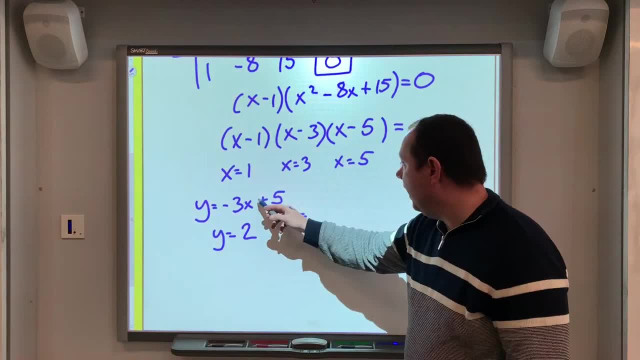 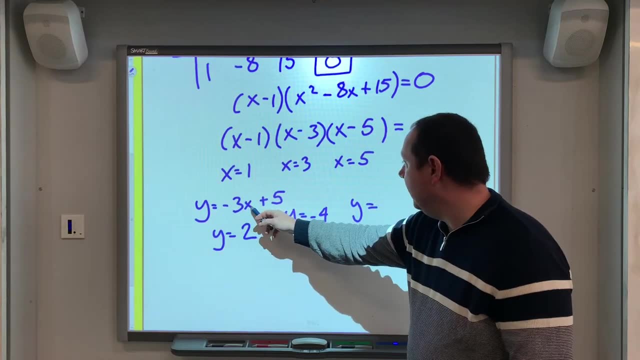 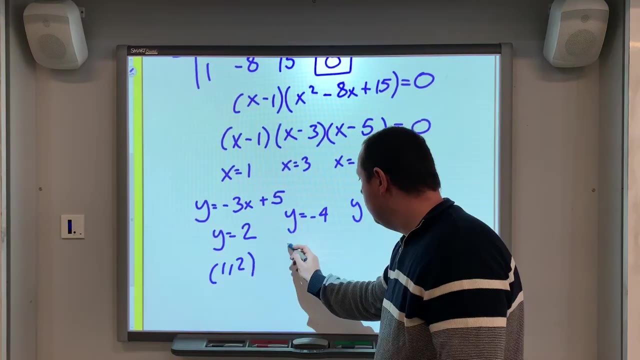 For this one, y equals minus 9, add 5,, which is minus 4.. And for the last one, y equals minus 15, add 5., Which is minus 10.. Our points are 1,, 2,, 3 minus 4, and 5 minus 10.. 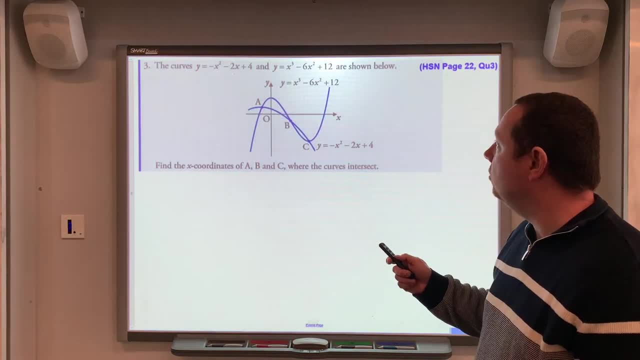 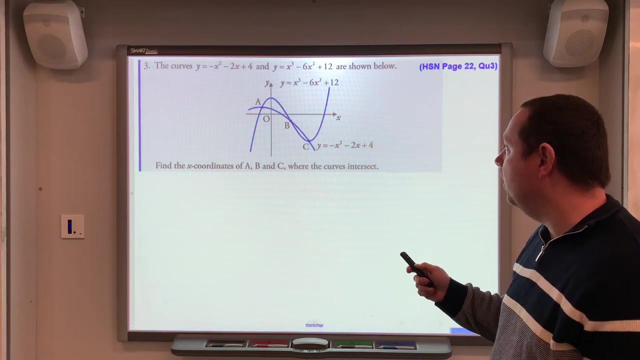 Example 3.. The curves- this one y equals and it's a quadratic- and this cubic are shown mobile. So you can see the cubic goes here and we've got a bit of the quadratic here Which would extend this way to make it for that one. 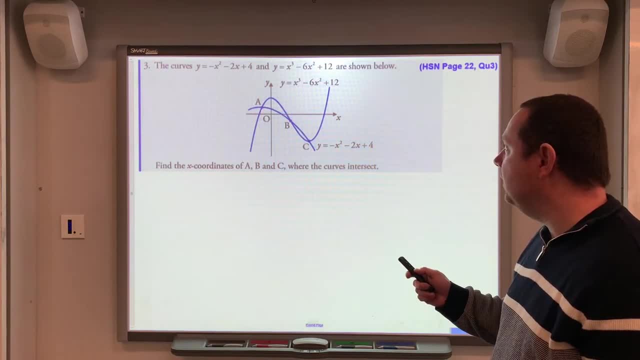 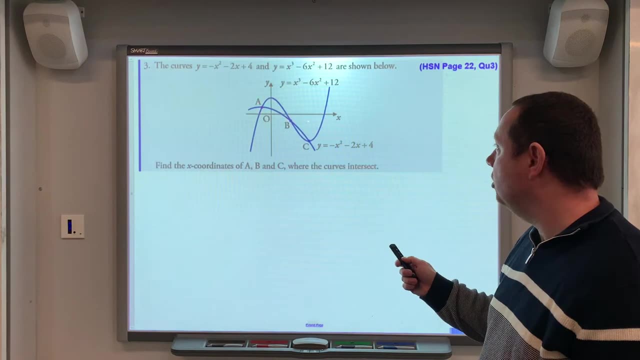 And we have to find the coordinates, just the x part of a, b and c. So you can see, here we've drawn us a picture, but it's asking us to find the points of intersection, because it's where the curves touch. 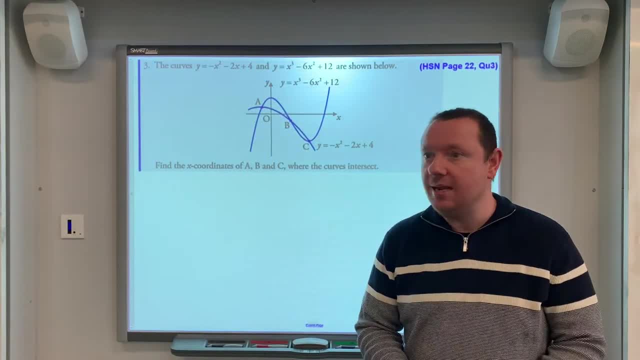 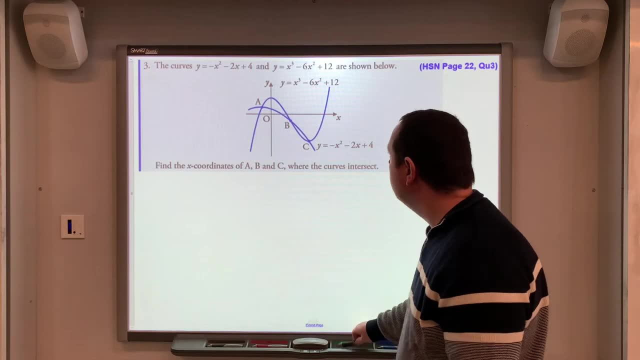 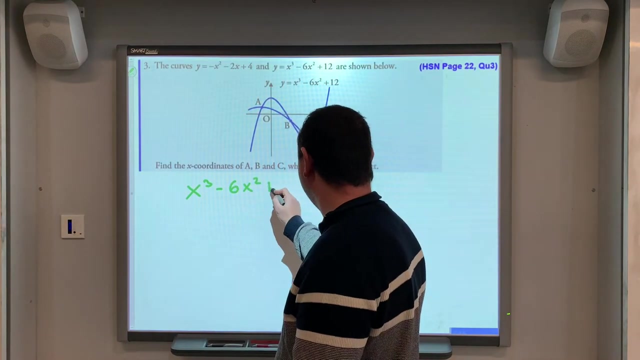 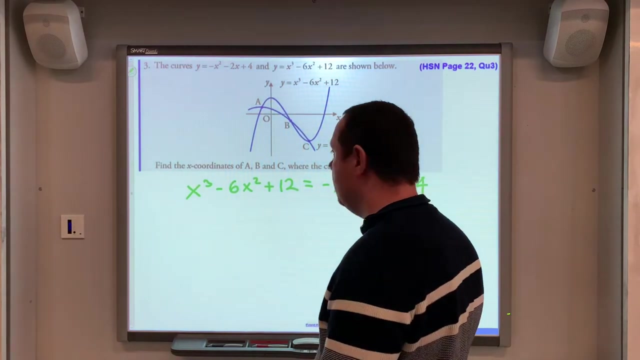 So we're just solving simultaneous equations, the same as usual. So we make this curve equal to this curve. We both say: y equals x cubed minus 6x squared plus 12, equals minus x squared minus 2x plus 4, moving everything over to the left-hand side, 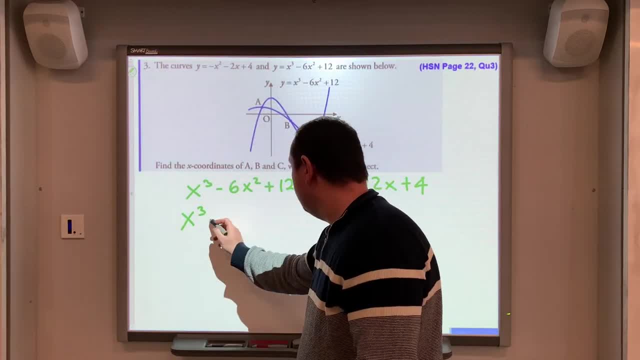 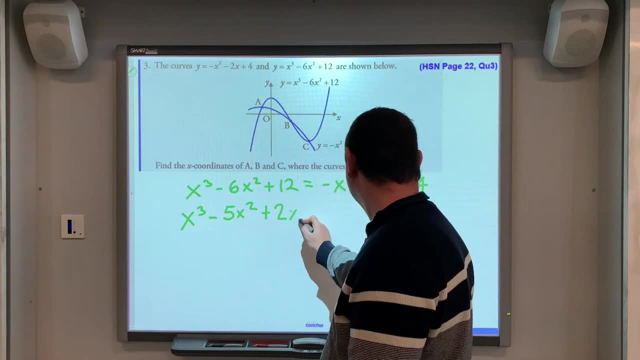 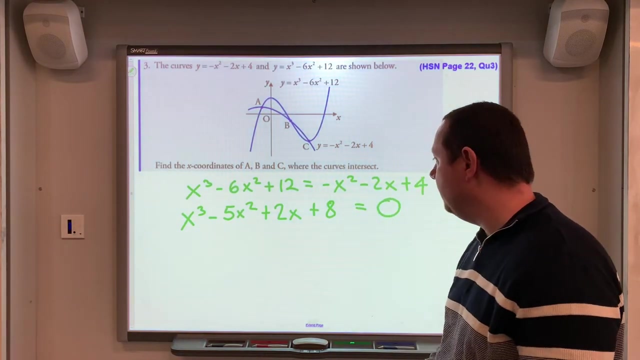 we've got x cubed minus 5x, squared plus 2x, and then 12, take away 4, is plus 8, and this equals 0, because everything's moved to the left-hand side. As per usual, we've got a cubic to solve, so we need to find one factor. 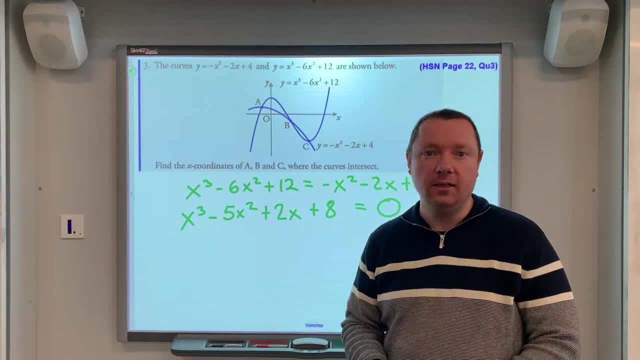 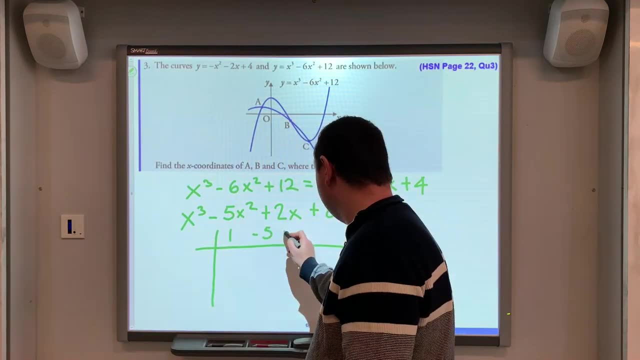 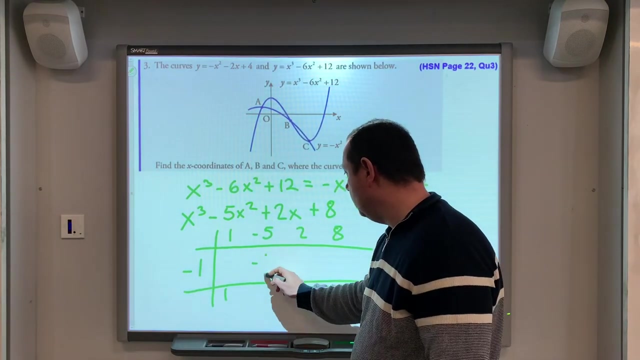 we're going to use synthetic division to factorise it to find the solutions 1, minus 5,, 2, and 8, substitute a minus 1 in 1, minus 1, minus 6, 6,. 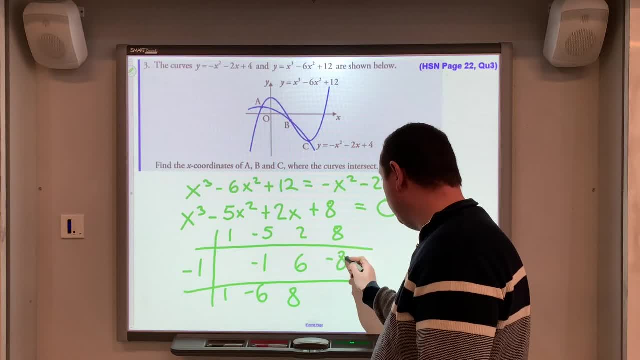 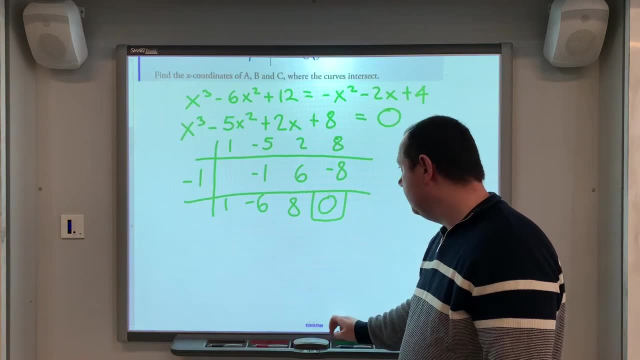 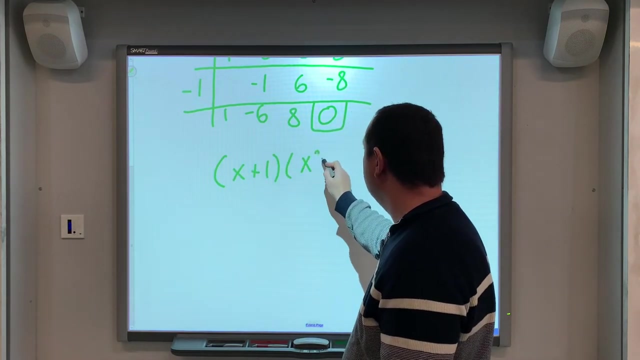 6 and 2 make 8, minus 8, we've got a remainder of 0, so that means that x add 1 is a factor. we've got x plus 1, and x squared minus 6x plus 8,. 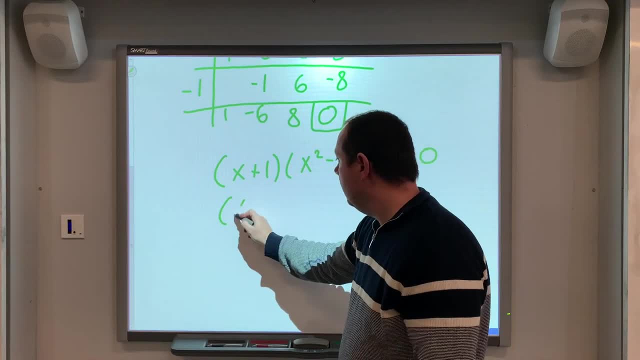 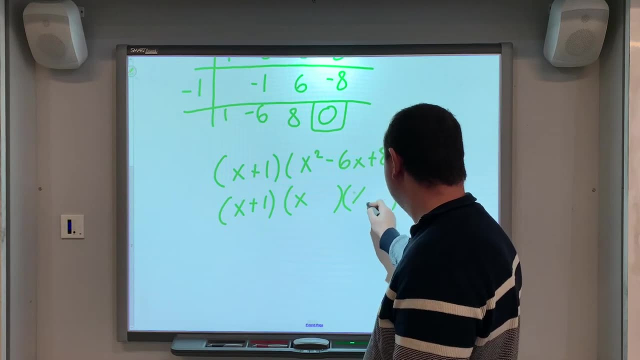 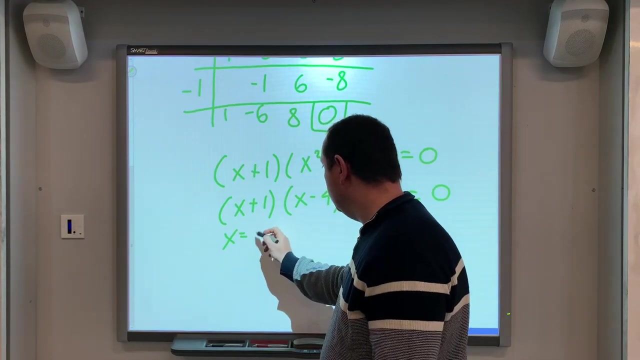 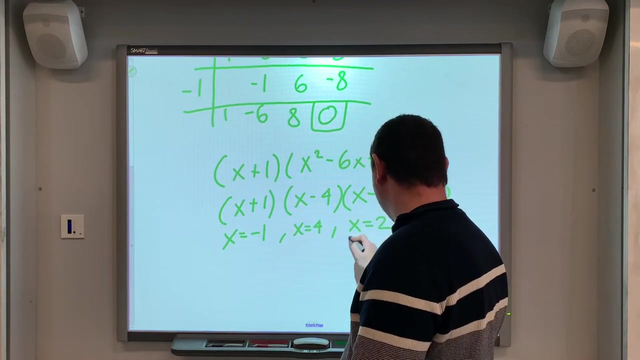 we've got 0,, 4 and 2, minus and minus x equals 1, so x equals minus 1, x equals 4, and x equals 2.. Now it was just the x part of the coordinate we wanted us to find. 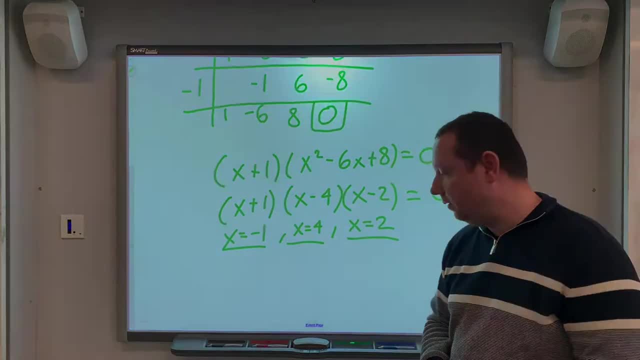 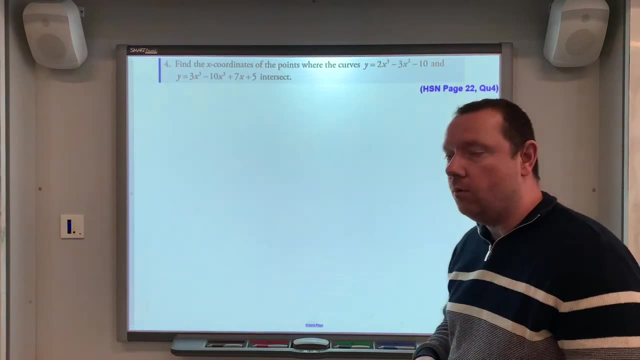 so we don't have to substitute that in to find the y part. we'll finish there. Find the coordinates of the points where the curves- and it's a cubic and another cubic intersect, So the word intersect or meet. solve them simultaneously. 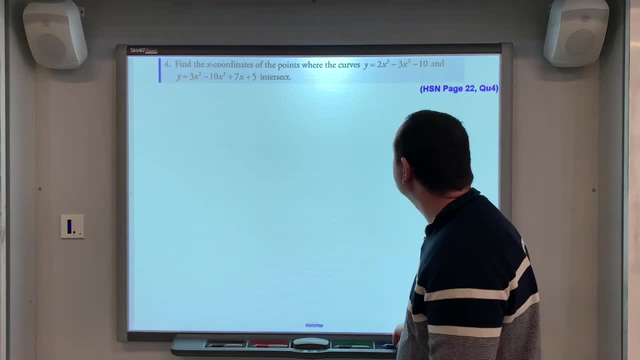 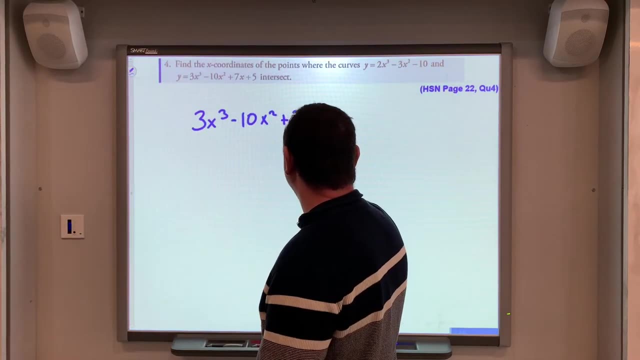 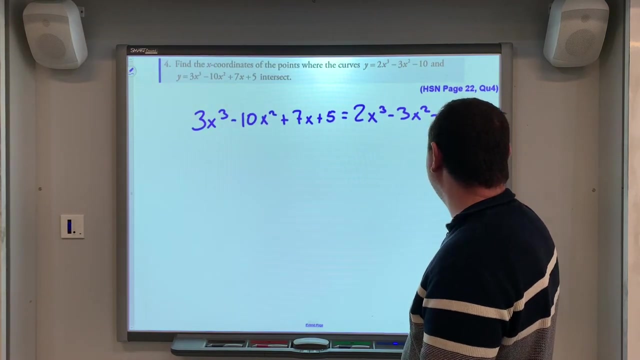 Constantly the same thing. So we've got 3x cubed minus 10x squared plus 7x plus 5, equals 2x cubed minus 3x squared minus 10.. Moving everything over to the left hand side is normal. 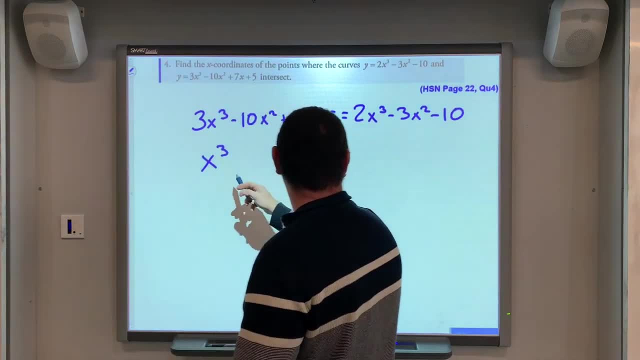 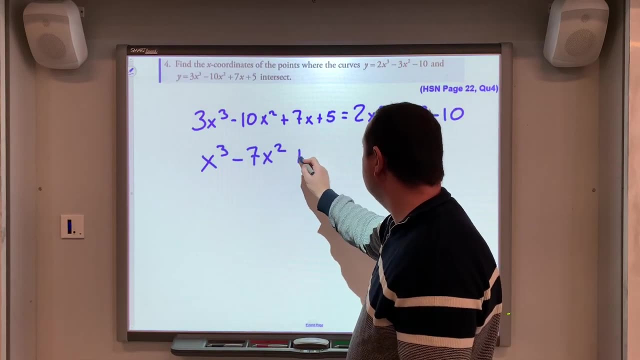 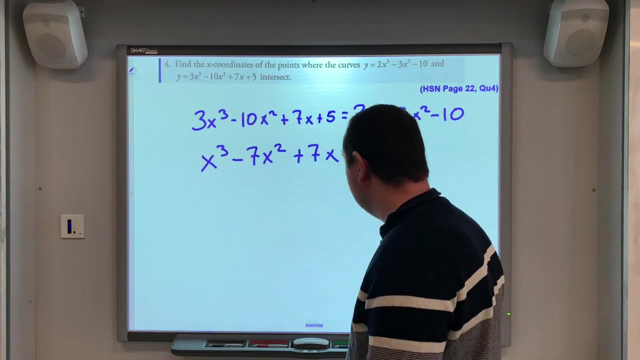 that gives us x cubed on this side Minus 10. add 3 is minus 7x. squared plus 7x plus 5, equals 2x cubed minus 3x, squared minus 10.. squared Only a 7x on this side, 5 plus 10 is 15 equal to 0.. We've got a cubic to solve. 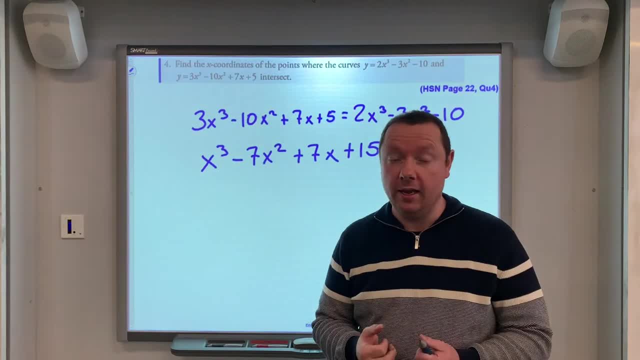 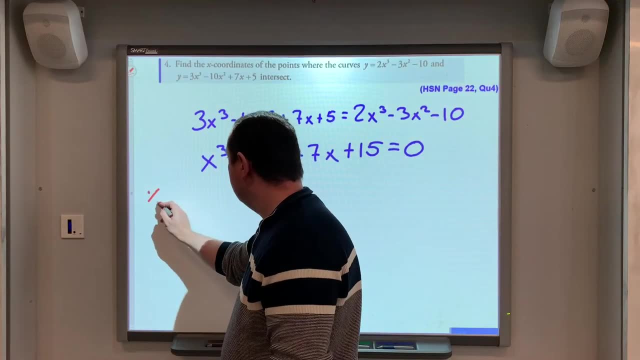 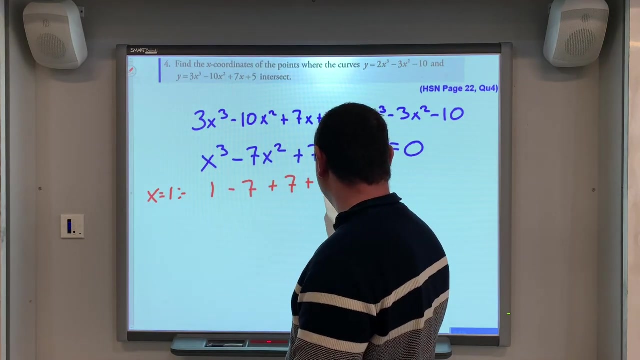 so, as per usual, we need to find one root just by trial and error and then use synthetic division to find the other roots. Let's actually show the whole process this time. Let's try one first, So we'll get 1 minus 7 plus 7 plus 15.. 1 plus 15 is 16, so that's not the. 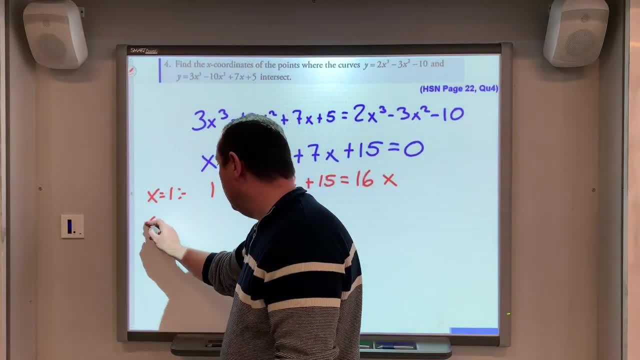 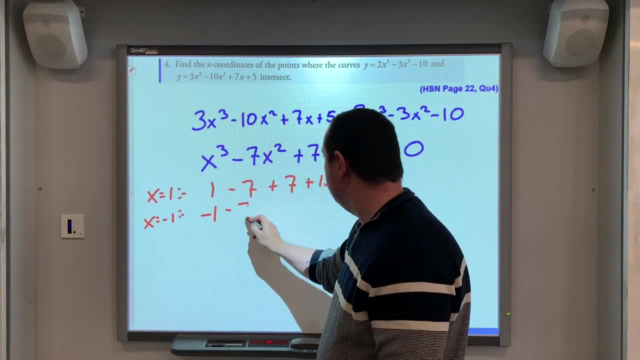 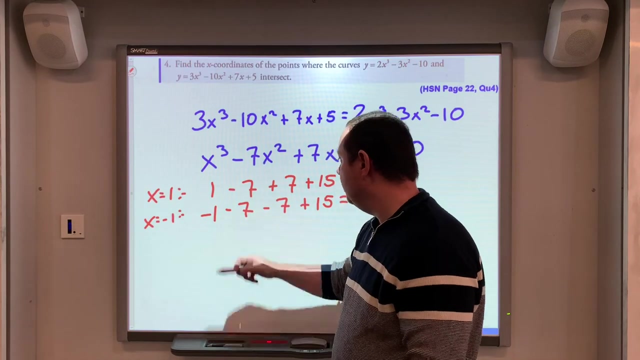 one I'm looking for because I need to get an answer of 0.. Let's try minus 1.. We'll get minus 1.. Minus 1 squared, take away 7.. Minus 7 plus 15.. 1 take away 7 is minus 8.. Minus. 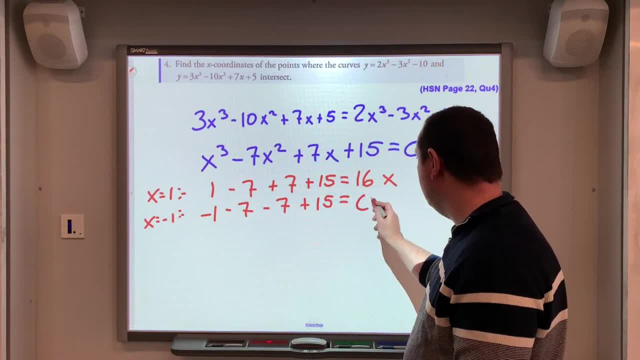 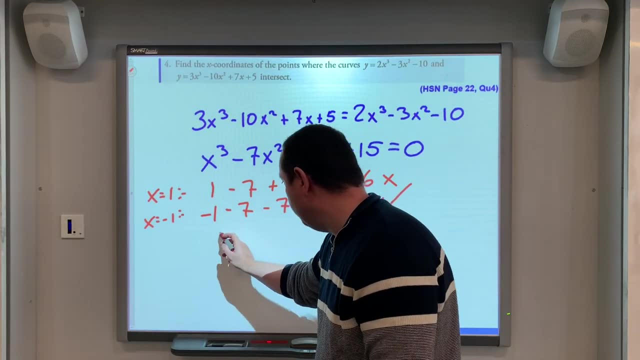 7 is minus 15.. Add 15 is 0.. So minus 1 is the one we want. We now know one factor x, add 1.. We can use synthetic division to find the rest. So we've got 1x cubed minus 7x squared. 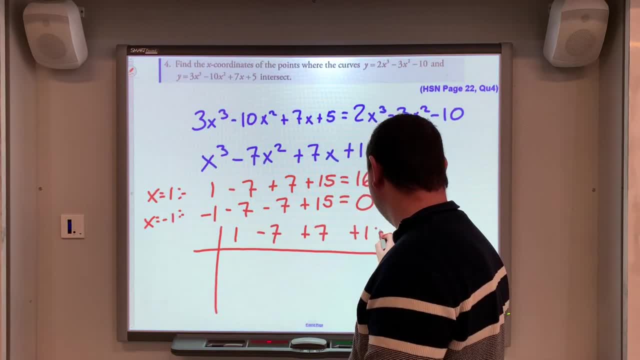 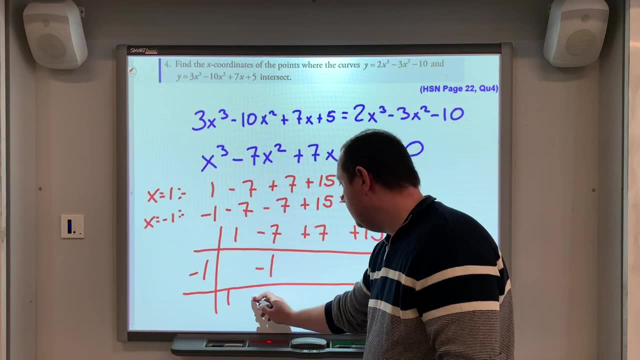 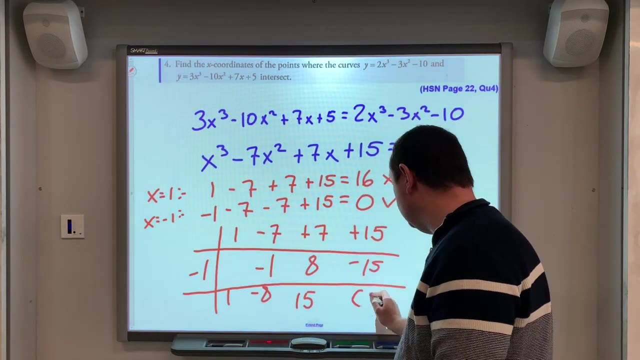 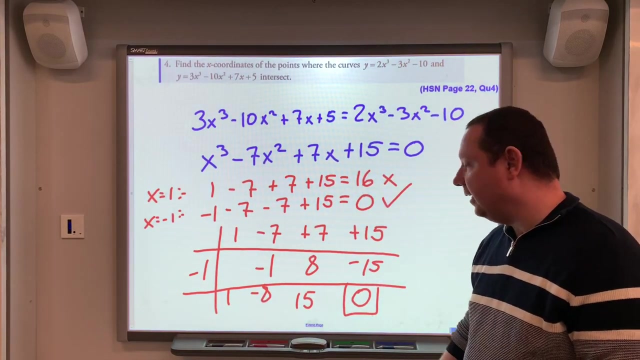 plus 7x plus 15, and we're substituting minus 1 in, So that gives us 1 minus 1 minus 8.. 8. 15 minus 15 and 0.. There is our other factor there: x squared minus 8x, add 15.. So we've 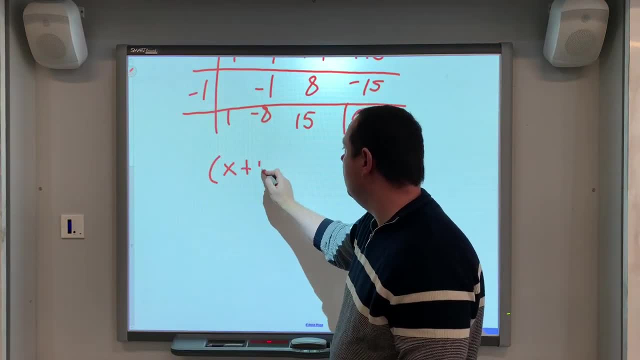 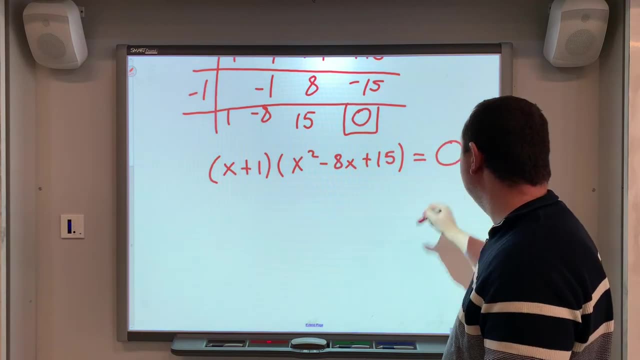 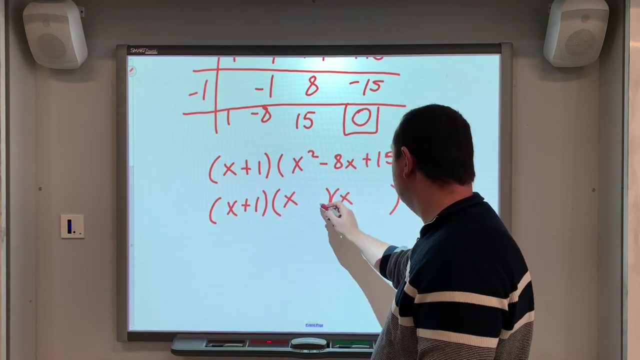 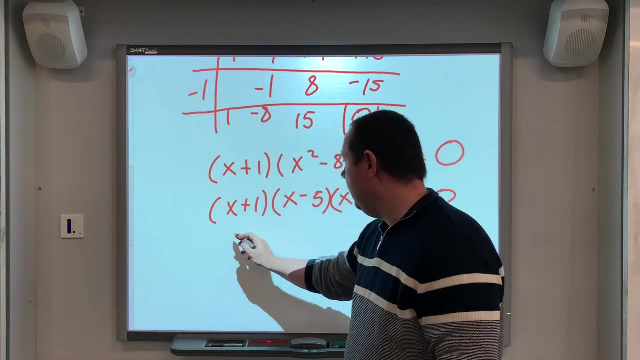 got. we've substituted minus 1 in, So x plus 1 is the factor and then we'll factor x squared minus 8x plus 15.. So this will then be equal to 0.. x and x, 5 and 3 make 8 and 15 when you times them Minus and minus 0.. x equals minus 1.. x equals. 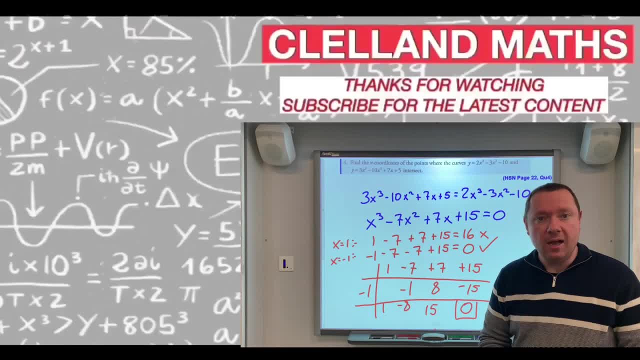 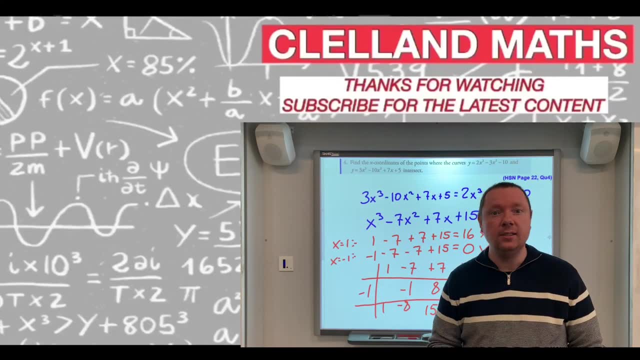 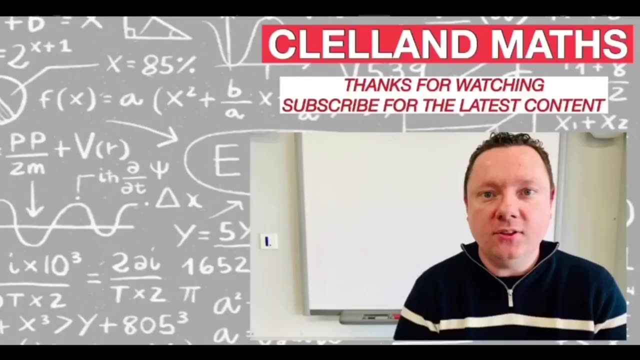 5. x equals 3.. This has been Clare Masters. Today we'll be looking at the point of intersection between curves, specifically cubics, quadratics or two cubics. Take care, stay safe and goodbye.